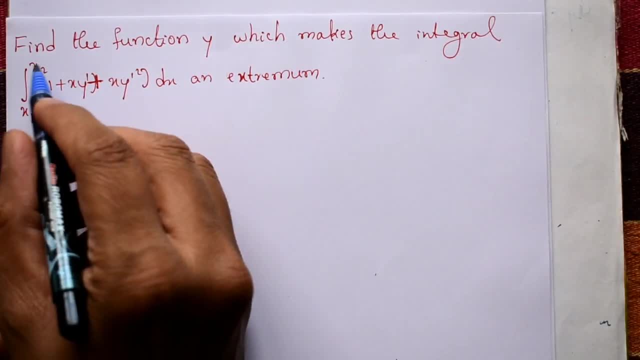 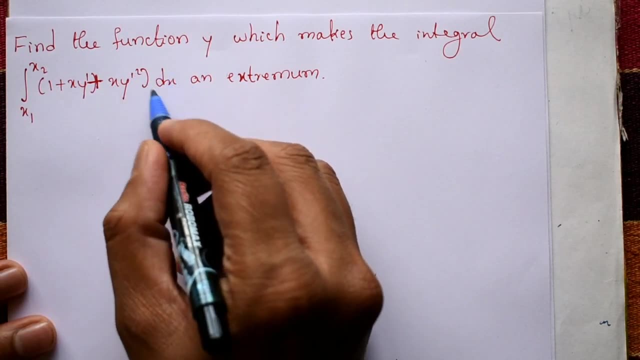 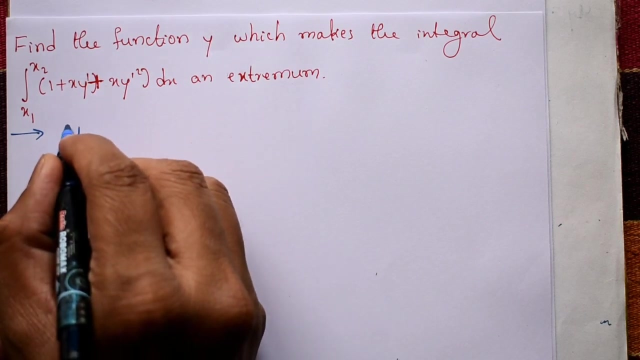 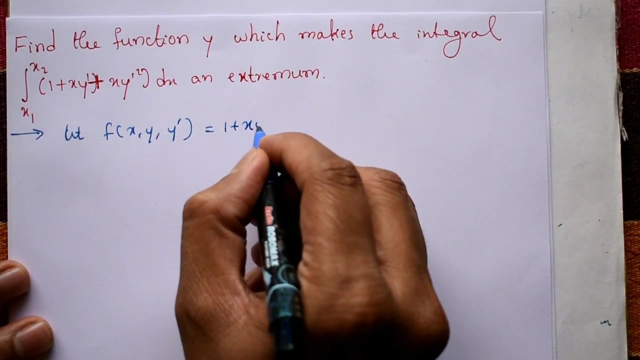 Find the function y which makes the integral integration. is given integration of x1 to x2, 1 plus xy dash plus xy dash, whole square with respect to x and xgmo. Okay now, this function is very simple Example. let now consider this part is a f of xy y dash, that is, 1 plus xy dash. 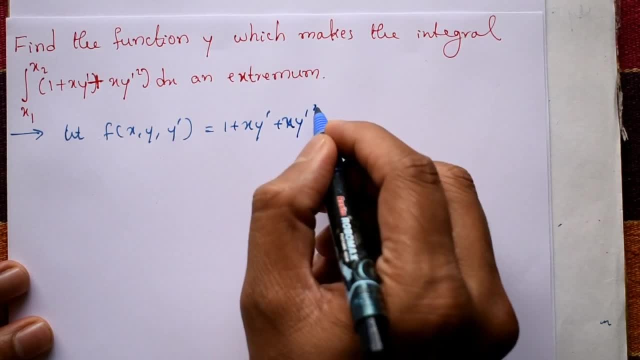 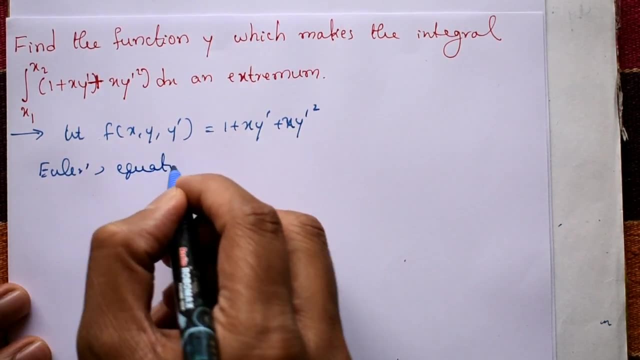 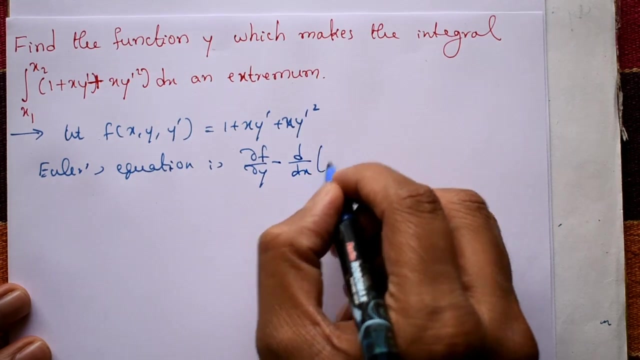 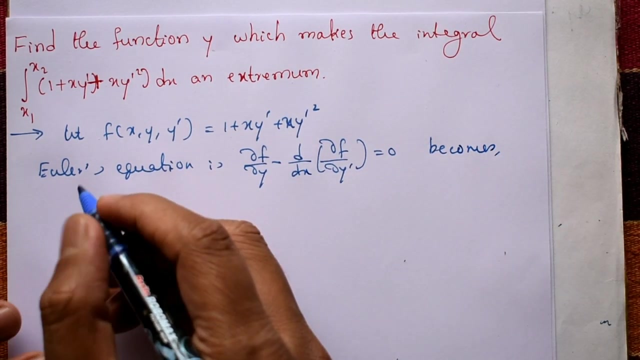 plus xy, dash whole square. Okay, now we are using a Euler's equation. Euler's equation is dou f by dou y minus d by dx, into dou f by dou y, dash that equal to 0.. This equation becomes Okay now. difference at f means this function with respect to y, no y variable means. 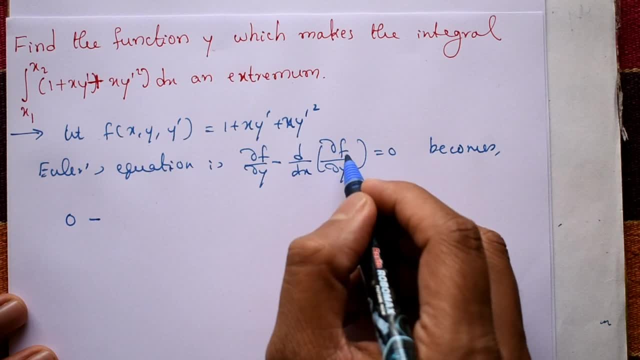 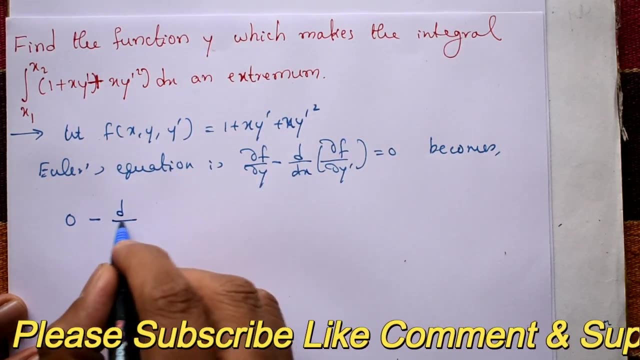 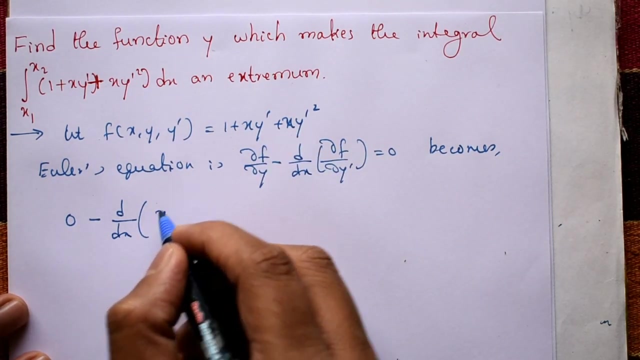 0.. Okay, now difference at f means this function with respect to y. no y variable means 0.. Now difference at f: this function with respect to y dash, only y dash, Now d by dx. this is as it is. dou means using PDE, x treated as a constant. Now x, y dash become 1, again plus x. as it is. 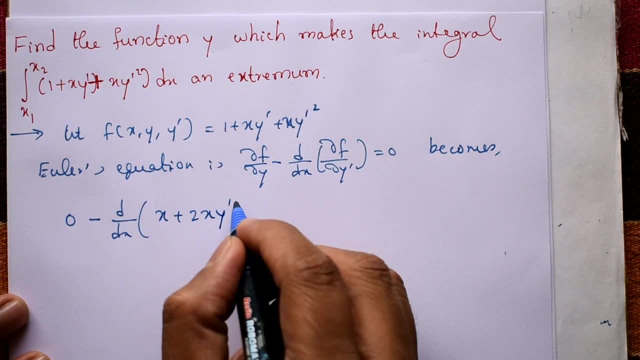 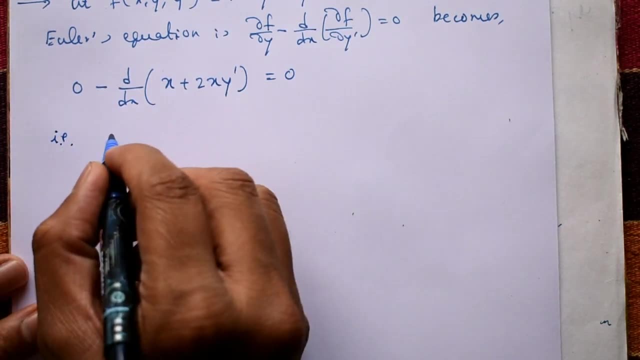 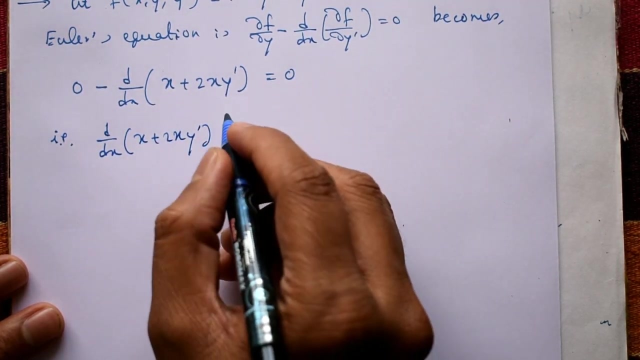 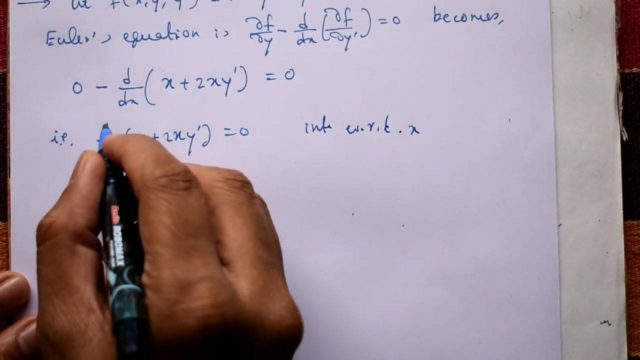 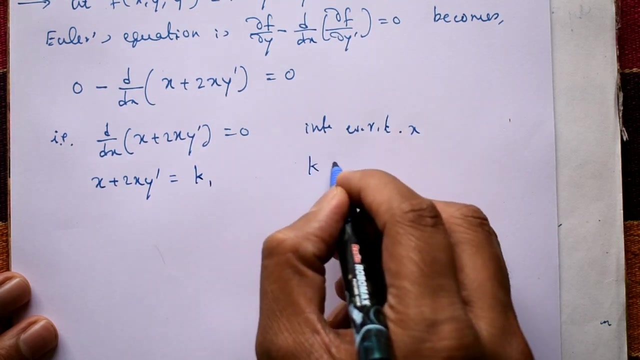 y dash whole square. differentiate, you get 2 into y dash that equal to 0.. Okay now, now that is, this equation becomes d by dx plus 2 x y dash that equal to 0.. Now integrate with respect to x. this is cancel. remaining x plus 2 x y dash that is equal to k1.. Now k1 is also. 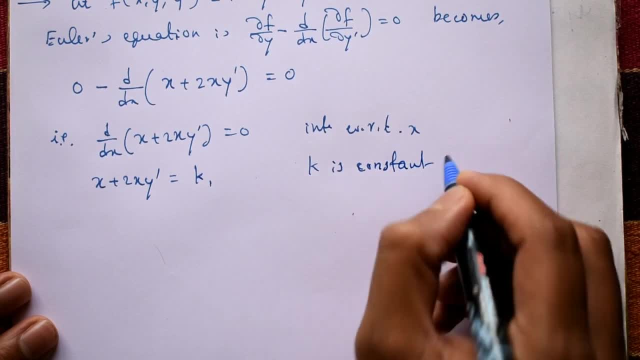 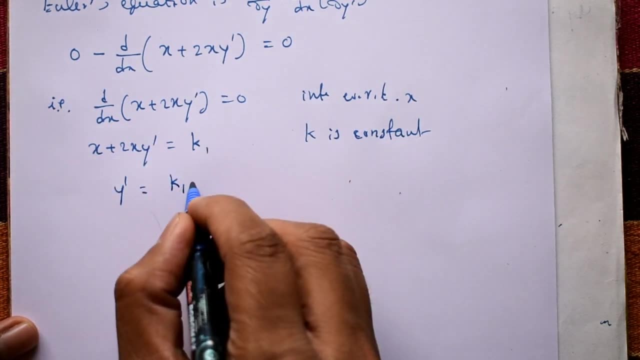 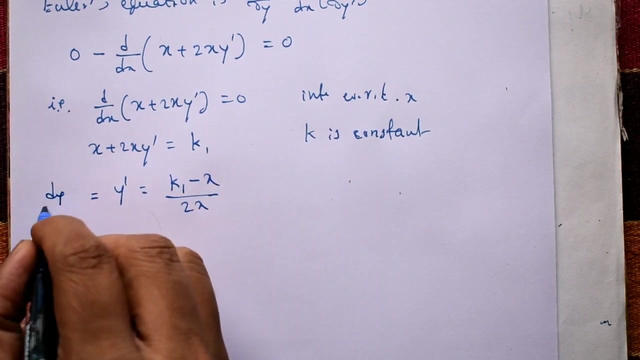 is a constant. Okay, now y dash is equal to now k1, x shift right hand side is minus x, remaining 2: x shift in denominator. k1 minus x divided by 2, that is a y dash. Y dash means first order d by dx. 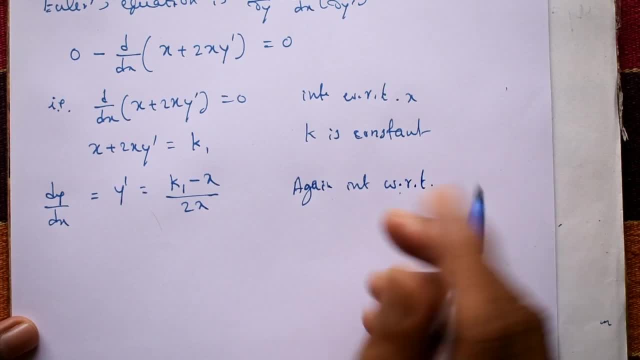 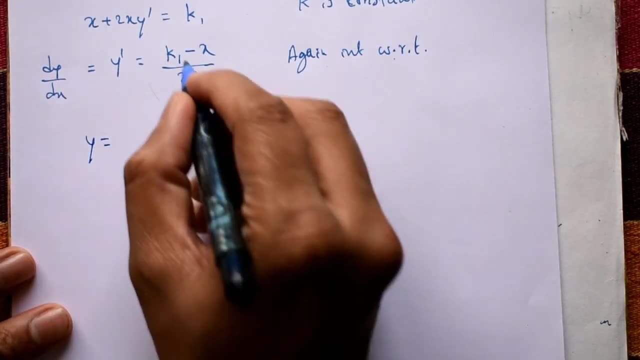 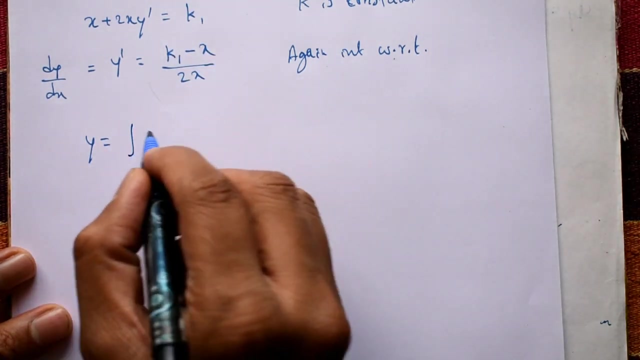 Again integrate. Okay, once again integrate. with respect to x. This equation becomes d by dx, become y is equal to: it is a two terms: k1 by 2 x or minus x by x. Let us take a separate integration of k1 by 2 x with respect to x. minus sign integration.